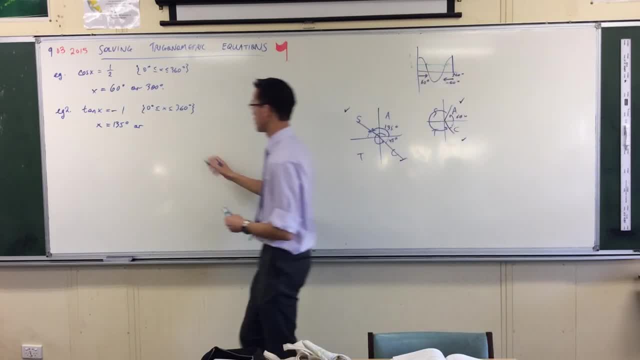 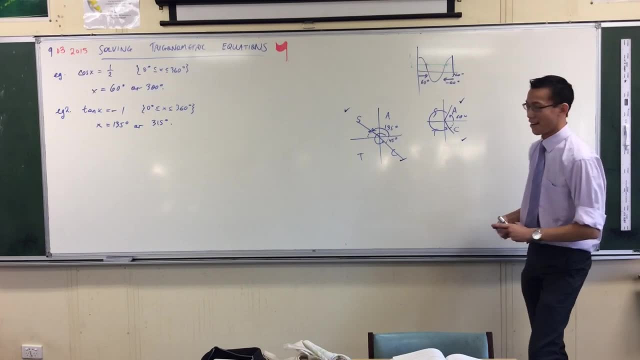 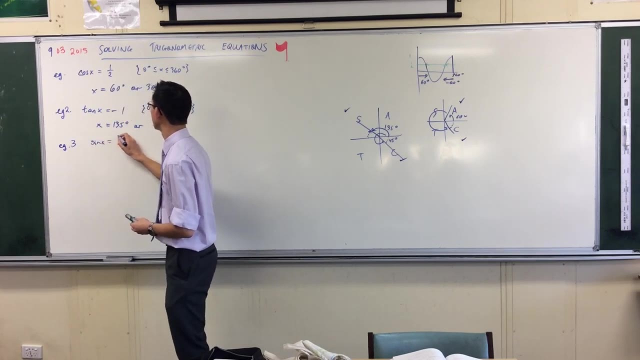 So what's that size? 315.. Very good, Okay, there you go. That's it. Nothing too dramatic. Okay, a third example. This time I'm going to switch it up a little bit. Let's go here. Oops, that's wrong. 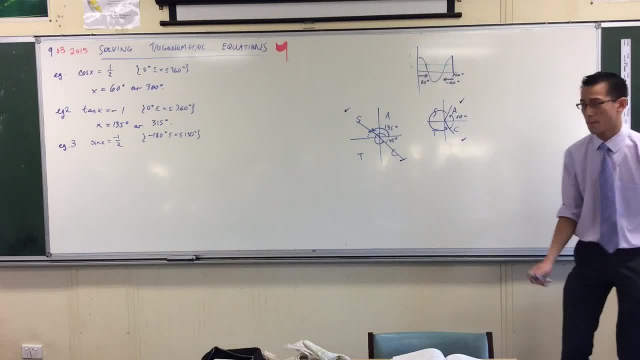 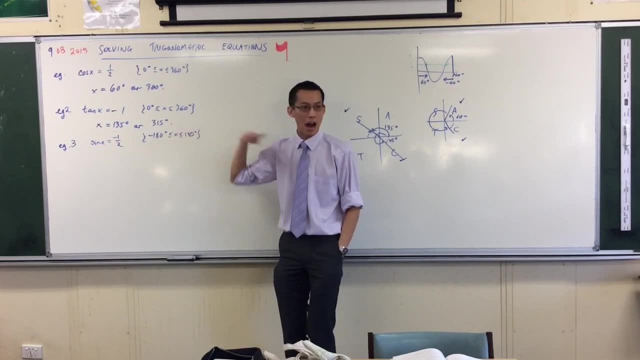 Okay, So I've changed the domain here and I'm pointing it out to you. You won't always get it pointed out to you, You have to look for yourself. okay, Now I will say like we went straight to the quadrants here. 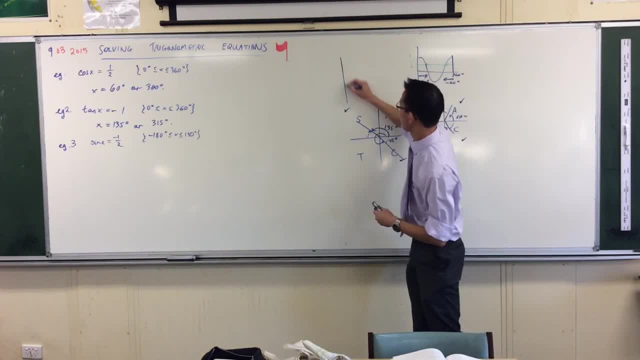 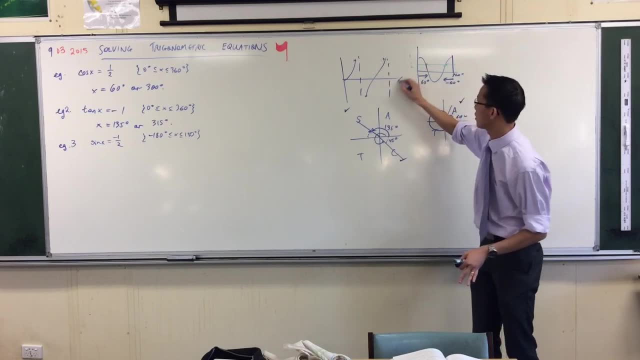 I'll just quickly draw what's happening for this second one. right, This was tan. What does tan look like from 0 to 360?? You're going to go up here asymptote, down asymptote And you've got your two copies of tan, because tan is periodic: every 180 degrees, right? 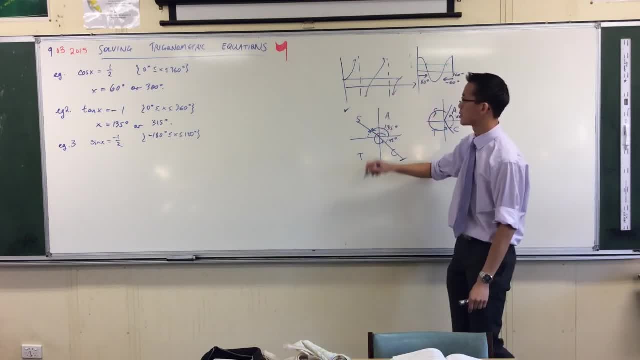 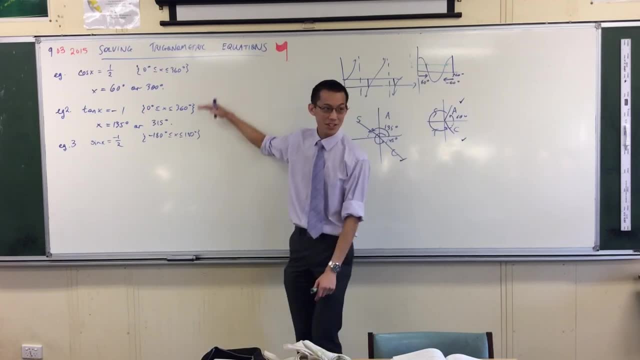 Where are our two solutions? Minus 1 is going to be somewhere down here, isn't it? So there's your 135, and there's your 315.. All happy times. okay, Now I've been kind of agnostic with these ones as to which approach you use. 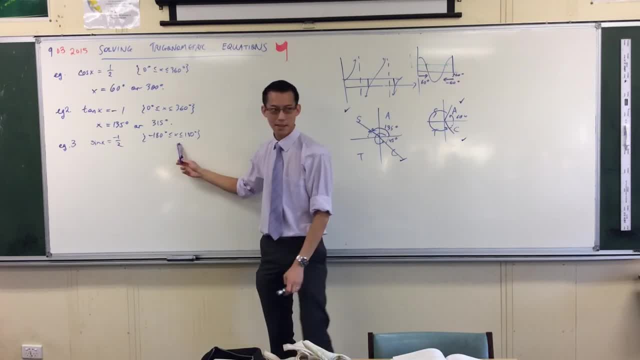 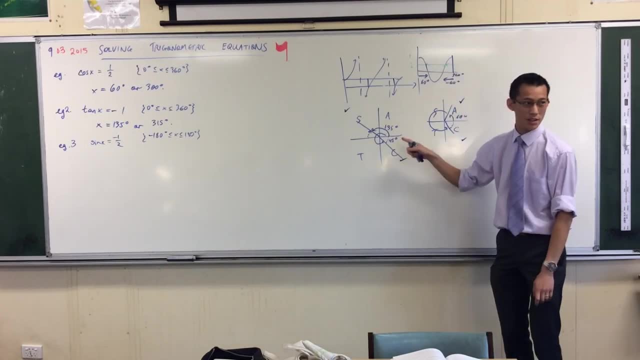 They're roughly equivalent. okay, But here, here, I think, is where the graphical method really starts to take over. okay, Because I could look at this in terms of quadrants, right, Except if I think about this domain here, right. 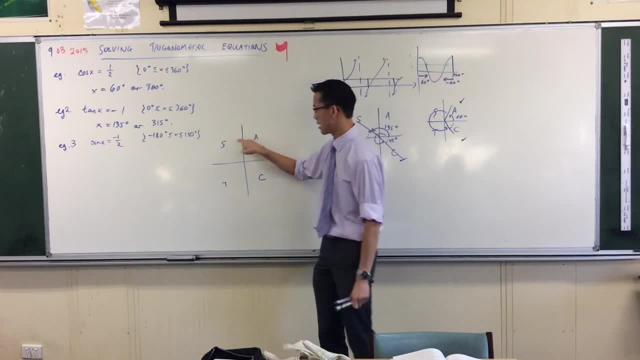 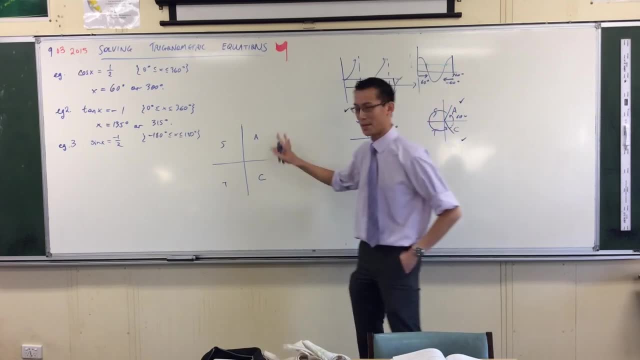 We usually think of this as 0 to 90,, 90 to 180,, 180 to 270, and 270 to 360.. And that's fairly natural and you should think about it that way, But that way won't work when you're looking at this domain. 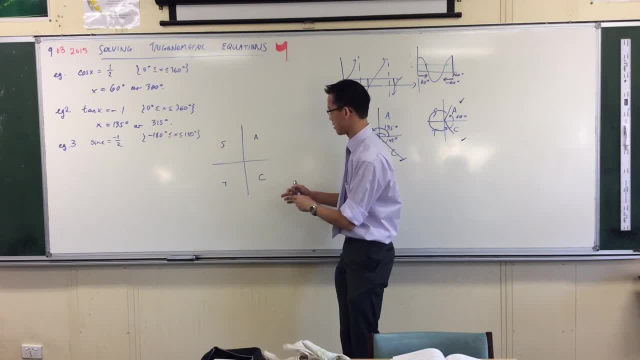 Will it right? Instead, you've got to think: okay, this is going to be 0 to 90, like before, This is 90 to 180, like before, But this is not 180 to 270, because 180 to 270 is not in your domain. okay. 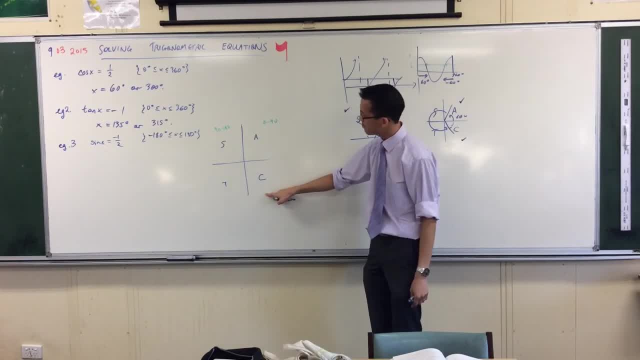 And neither is 270 to 360.. Instead, how would you suggest I write this? How do I do this? This is going to be negative 90 to 0.. And this is negative 180 to Negative 90.. Negative 90..